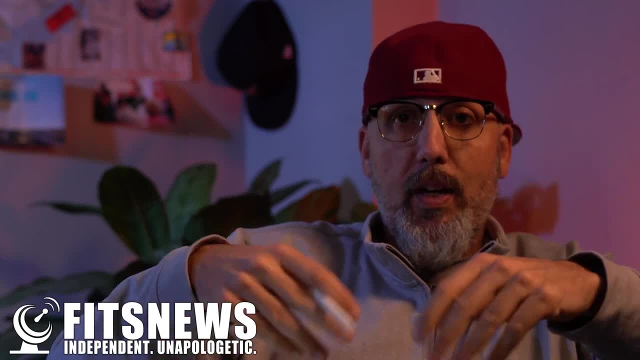 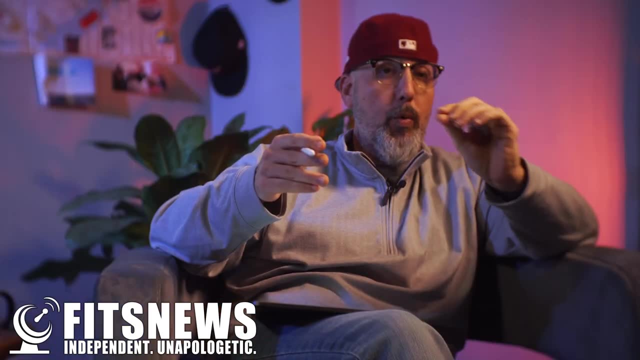 politicians hold up their tweets and their press releases touting that they did this or that to create jobs. Well, that's actually not the number you should be looking at, because that only tells a small fraction of the real story. The unemployment rate only tells a small part of the story, because 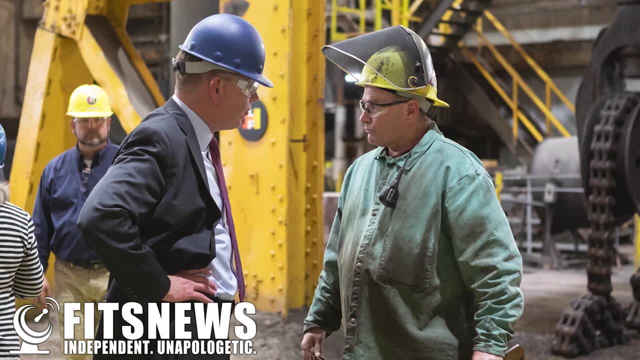 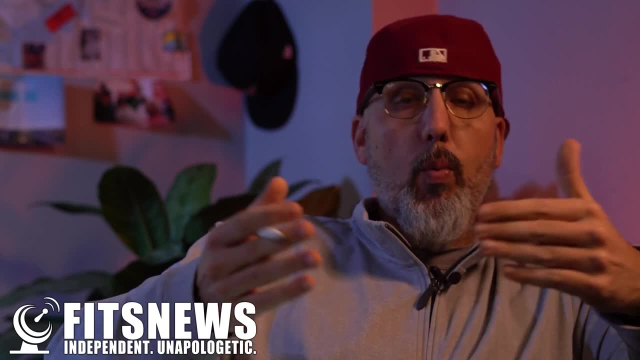 it's only a small part of the workforce. The workforce is actually about two and a half million people in South Carolina and that's the number we should be looking at. That number is a percentage of our working age And I know I've already bored you to tears, but let me try to explain it. Every month, the US 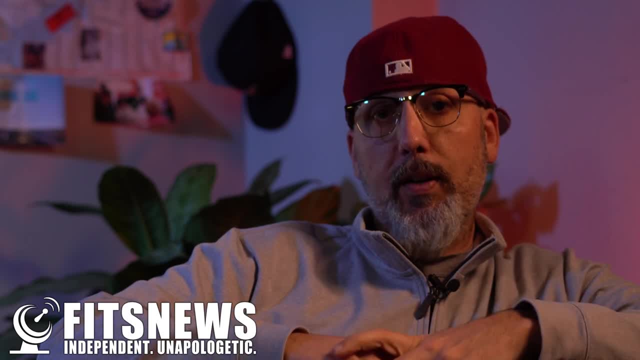 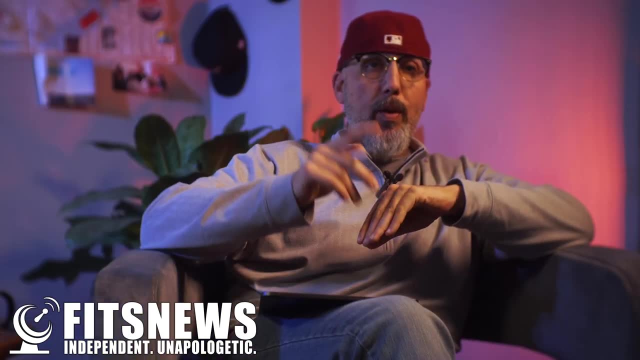 Department of Labor releases monthly unemployment data for the state of South Carolina and all the other states. South Carolina typically does well on the unemployment front, but doesn't perform well on the number that really matters, which is labor participation. So let me explain to you what labor 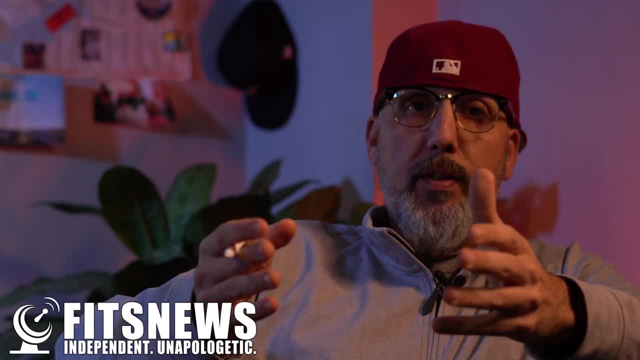 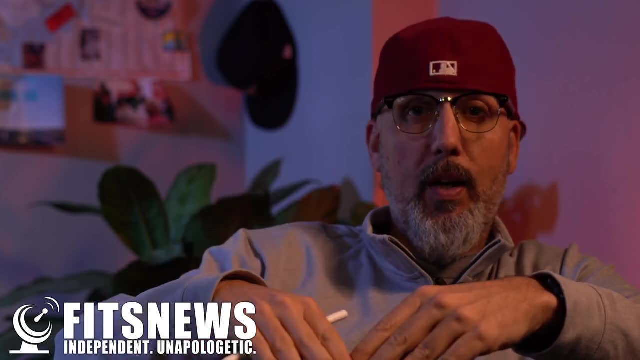 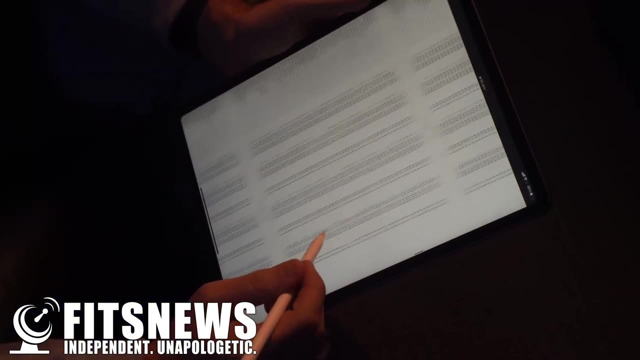 participation is. It's the percentage of the workforce that should be working that actually is working, And in South Carolina that number has historically been the highest And in South Carolina that number has historically lagged well behind the national average And in fact we're one of the bottom 10 states in the country. have been for years, In fact, pretty much since they started tabulating this data way back in 1976.. 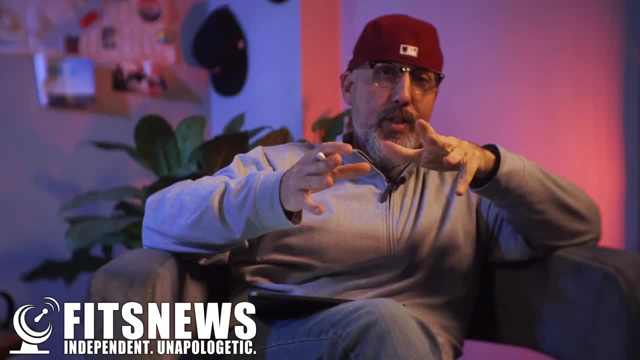 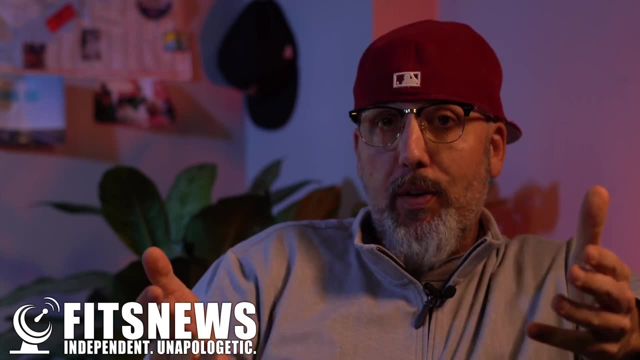 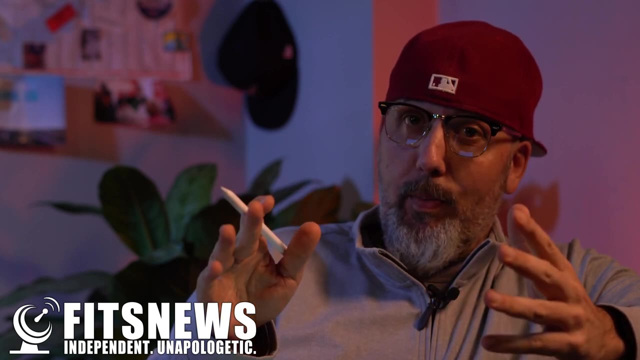 So, unlike the unemployment rate, which only tracks a small segment of the workforce, labor participation tracks the size of the workforce itself, which is what we should be looking at, And in South Carolina, the size of the workforce is consistently smaller than it is in other states, which is a problem. 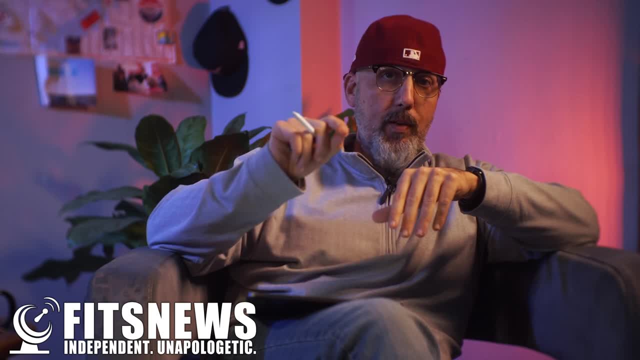 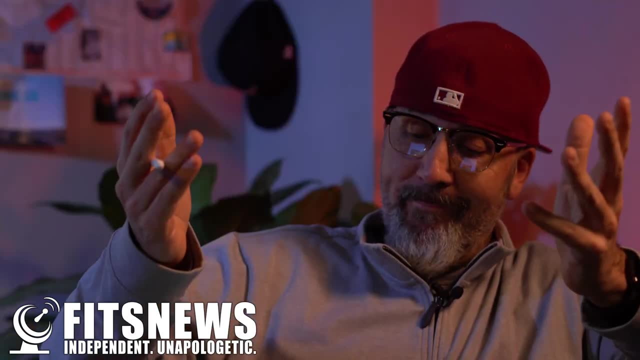 So let's do the math. This month, 4.2 million South Carolinians are of working age, meaning they should be part of the labor force. Now, how many of them are actually part of the labor force? 2.4 million, which means we have a labor participation rate of about 57.2 percent. 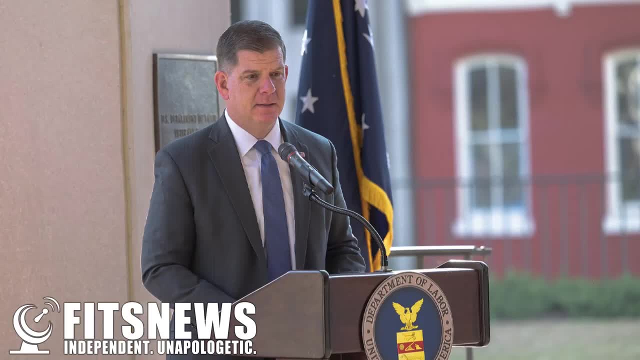 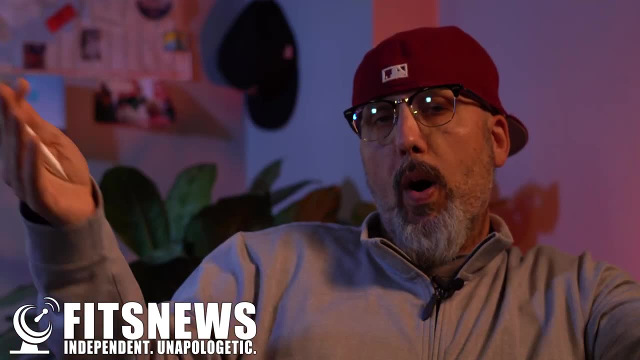 Now this is going to change when it's adjusted by the bean counters up at Washington. but that's about a level reading of what the rate is. So here's the question: Why do you not hear this data from the mainstream press? Why don't they focus on this? 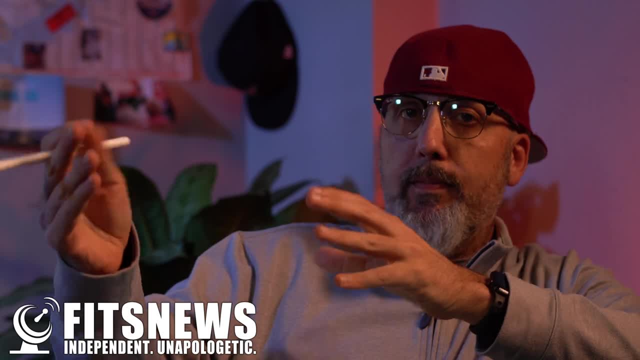 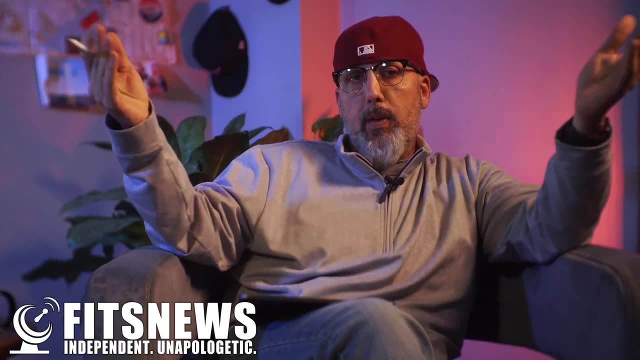 number. Why did they talk to you about the unemployment rate which, again, there's only one small percentage of the workforce and, again, whether it rises or falls really doesn't matter in the big scheme of things. I'll tell you a reason.